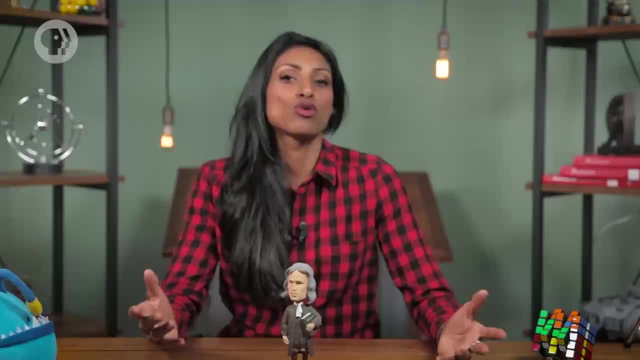 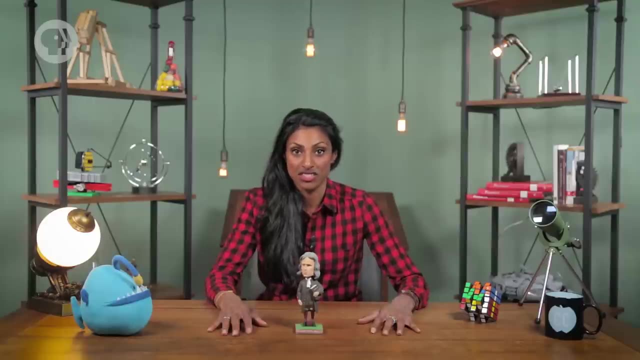 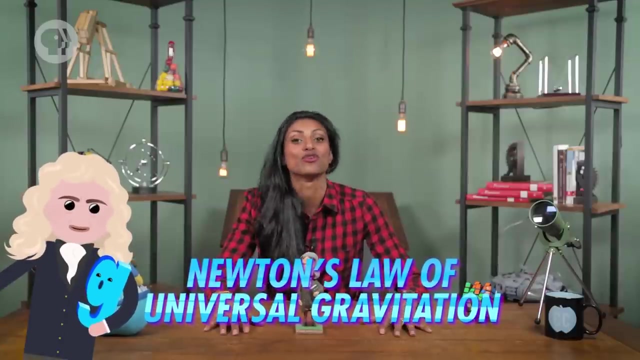 What they didn't know was that those two concepts were connected, Of course. just like with motion, we now know that there's a lot more to gravity than what Newton was able to observe. Even so, when it comes to describing the effects of gravity on the scale of, say, our solar system, Newton's law of universal gravitation is incredibly useful. 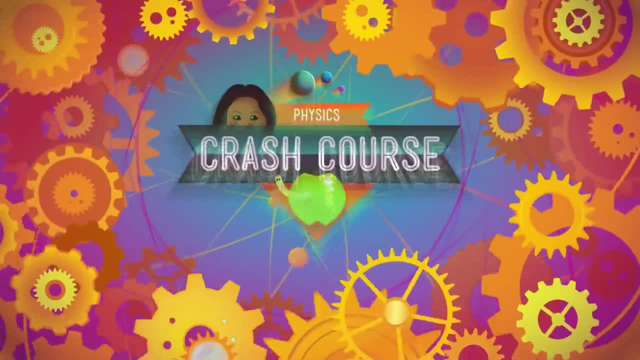 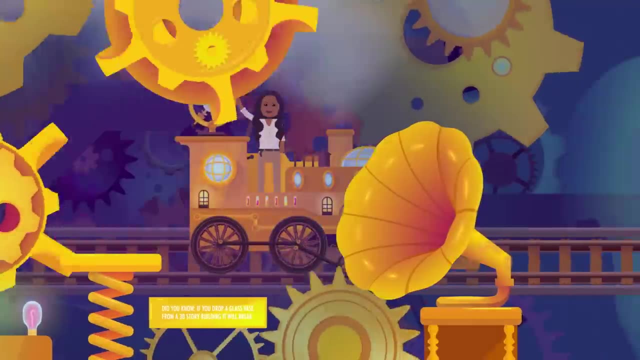 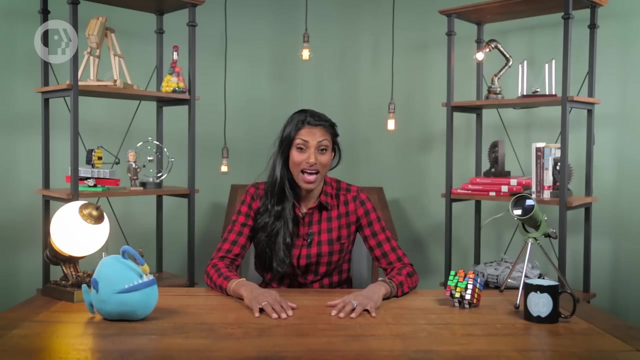 And it all started with an apple. Probably NISTENH boards Odds are. you've been told the story of Newton's apple at some point. The story goes that one day he was sitting under an apple tree in his mother's garden when an apple fell out of the tree. 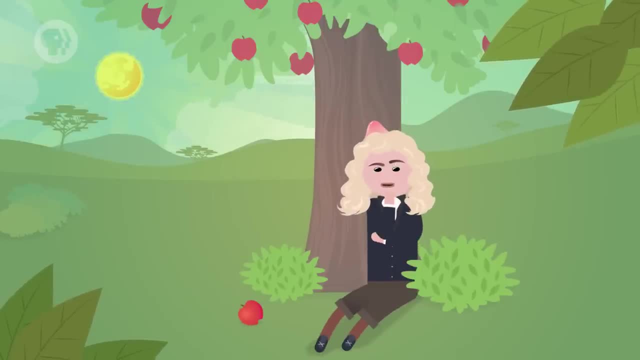 That's when Newton had his grand realization that something was pulling that apple down to Earth. And that led to another idea: What if the apple was pulling on Earth too? but you just couldn't tell, because the effect of the apple's force on Earth was less obvious. 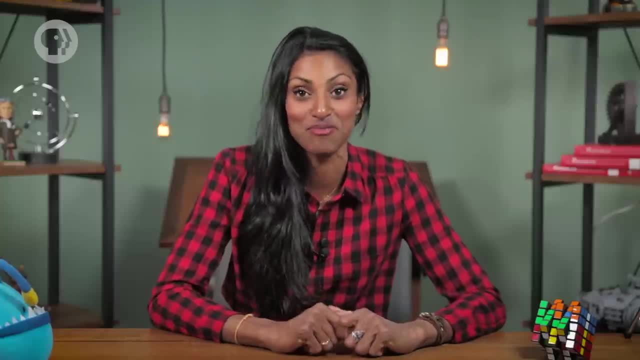 A few years later, Newton was sitting in the same garden when he had another stroke of inspiration: Hey tamam, This is it. The apple is pointing – The apple is pointing to – apple to the ground could affect things much farther from Earth's surface. Like the Moon. It was kind of counter-intuitive, because the Moon orbits Earth instead of crashing straight into the ground like an apple that falls off a tree. But Newton realized that the Moon was still being pulled towards Earth. it was just moving sideways so quickly that it kept missing. 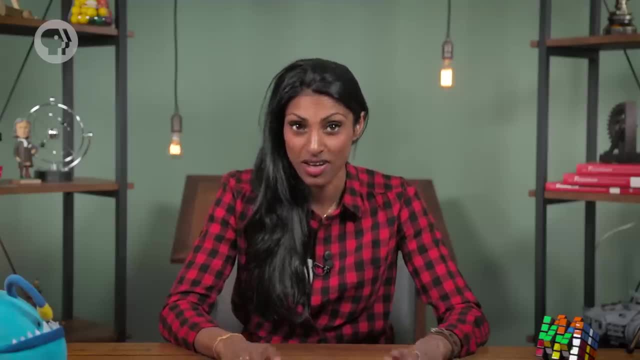 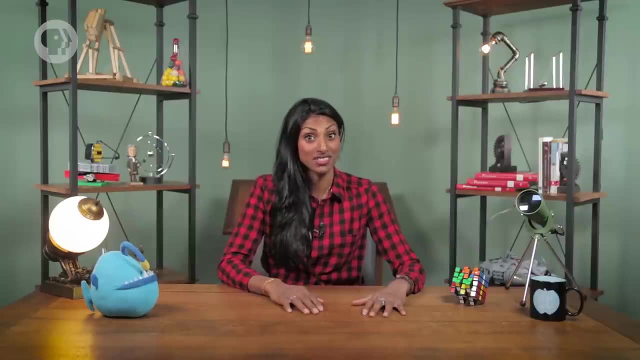 That was what was keeping it in orbit. If gravity was keeping the Moon in orbit, what if it affected the behavior of any two objects Like a planet orbiting the Sun? That's the official version of the story, the one Newton himself used to tell. 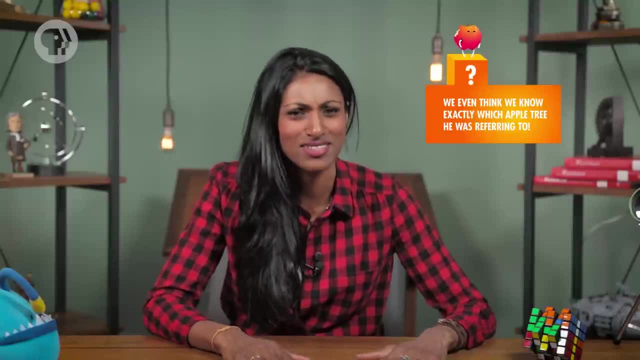 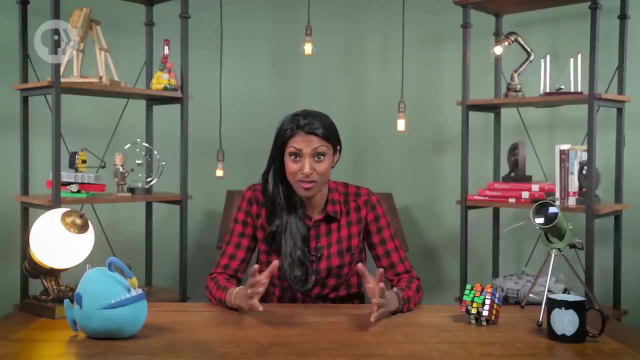 Most historians think he was embellishing, at least a little, but there probably is some truth to it, Whether or not the thing with the apple actually happened. Newton thought that his idea seemed promising, the idea that gravity might affect everything, including orbits of other planets. 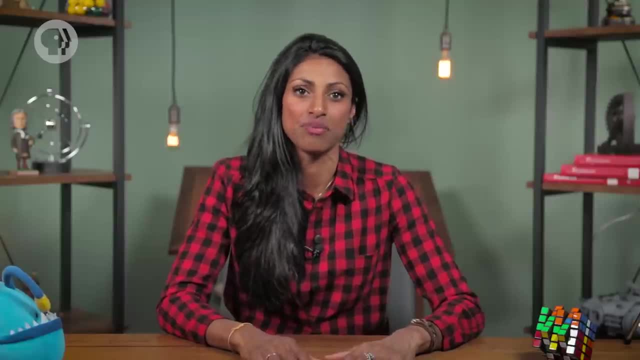 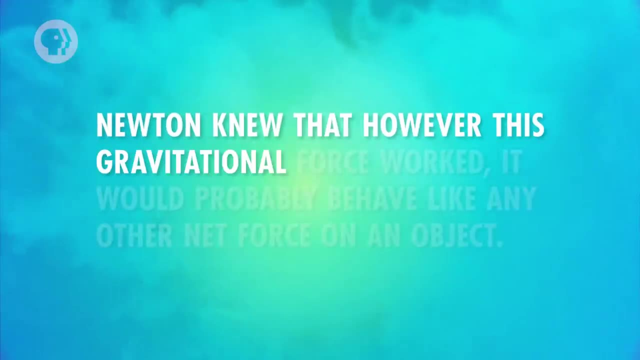 and moons. So he started looking for an equation that would accurately describe the way gravitational force made objects behave, Whether it was an apple falling on the ground or the Moon orbiting Earth. Newton knew that, however this gravitational force worked, it would probably behave like any other net force. 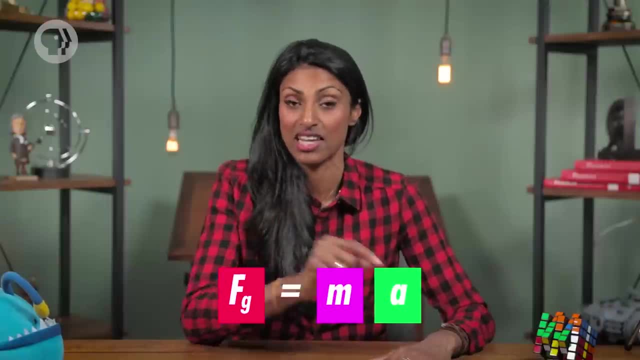 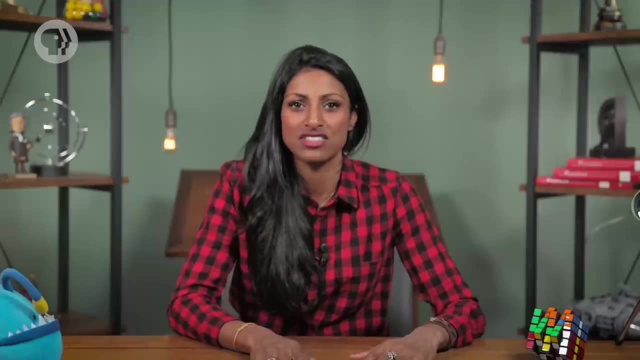 on an object, It would be equal to that object's mass times its mass. The mass part was easy enough – it would just be the mass of an apple Or the Moon. It was going to be a little harder to figure out the factors that were affecting the acceleration. 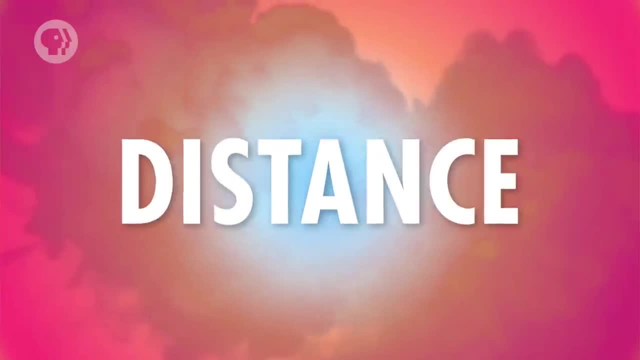 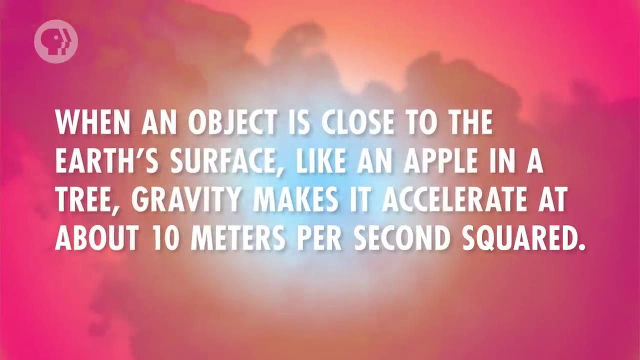 part of the equation. The first thing Newton realized he'd have to take into account was distance. When an object is close to the Earth's surface, like an apple in a tree, gravity makes it accelerate at about 10 meters per second squared. 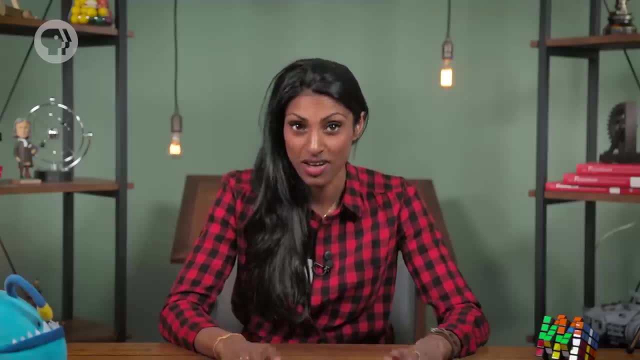 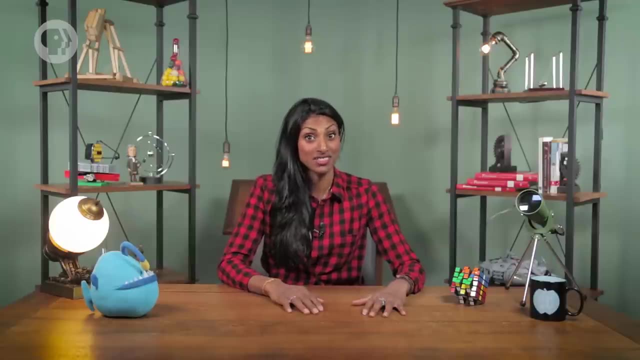 That was what was keeping it in orbit. If gravity was keeping the Moon in orbit, what if it affected the behavior of any two objects Like a planet orbiting the Sun? That's the official version of the story, the one Newton himself used to tell. 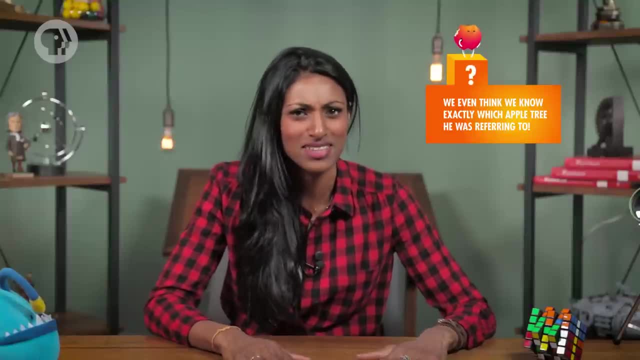 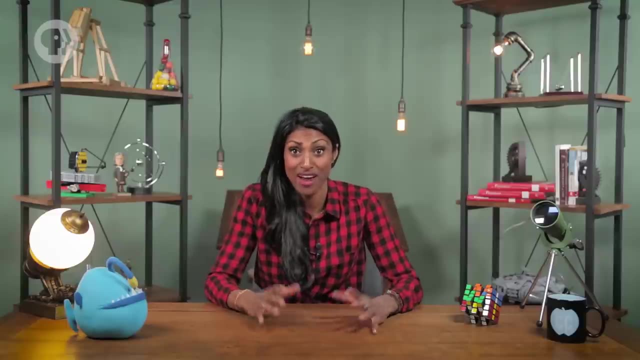 Most historians think he was embellishing at least a little, but there probably is some truth to it, Whether or not the thing with the apple actually happened. Newton thought that his idea seemed promising – the idea that gravity might affect everything, including orbits of other. 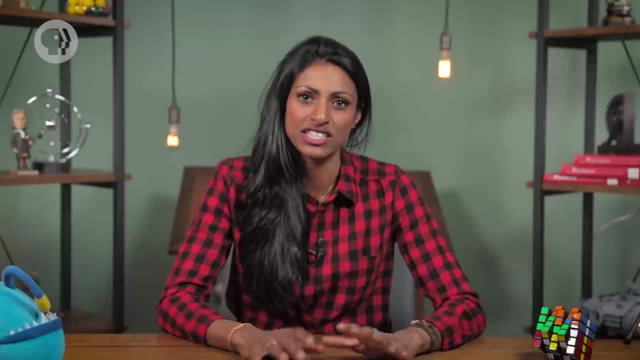 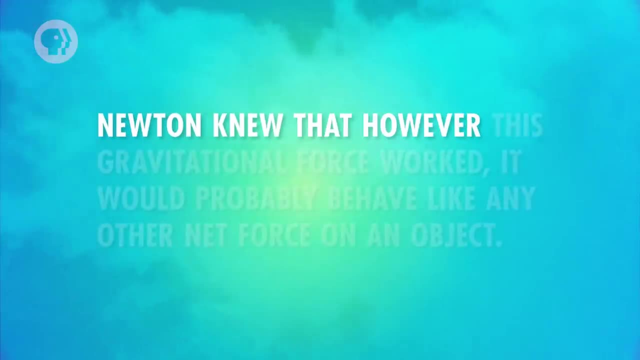 planets and moons. So he started looking for an equation that would accurately describe the way gravitational force made objects behave, Whether it was an apple falling on the ground or the Moon orbiting Earth. Newton knew that however this gravitational force worked, it would probably behave like any other net force. 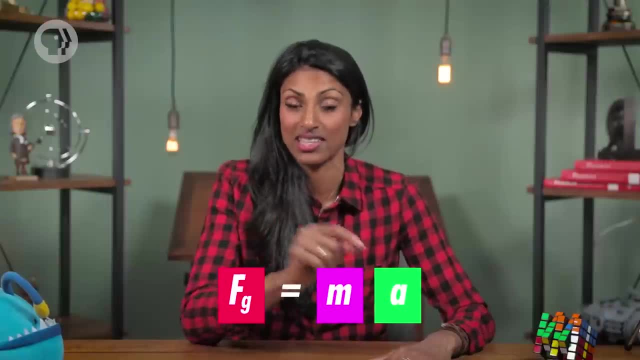 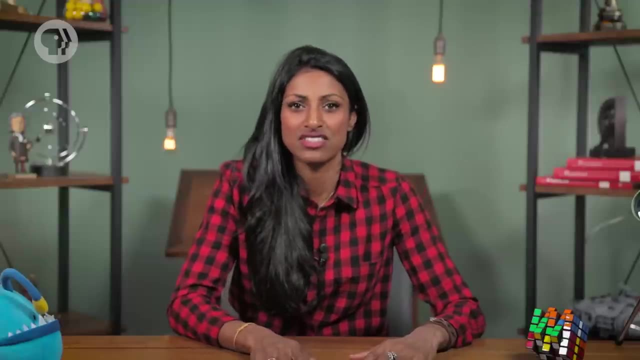 on an object, It would be equal to that object's mass times its mass. The mass part was easy enough – it would just be the mass of an apple Or the Moon. It was going to be a little harder to figure out the factors that were affecting the acceleration. 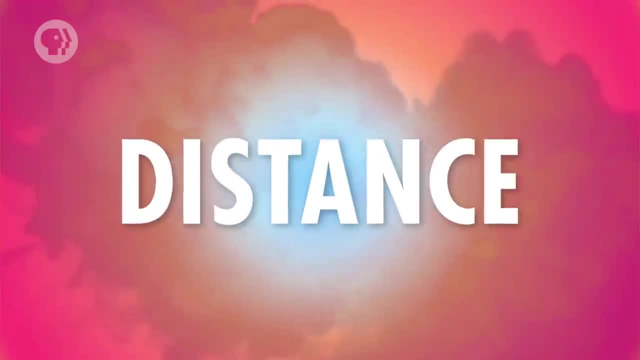 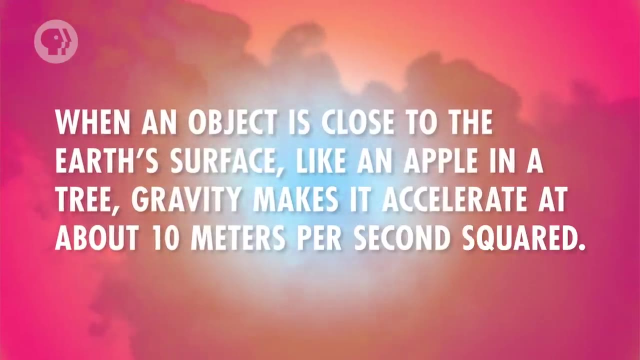 part of the equation. The first thing Newton realized he'd have to take into account was distance. When an object is close to the Earth's surface, like an apple in a tree, gravity makes it accelerate at about 10 meters per second squared. 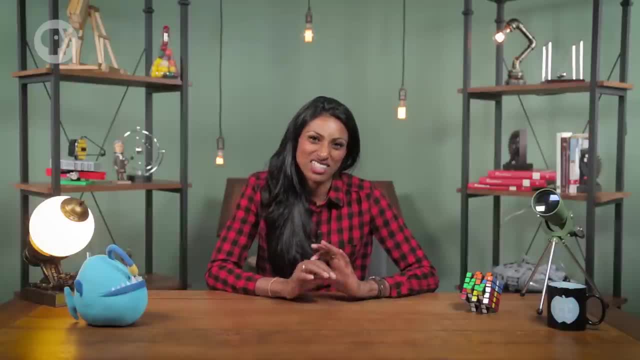 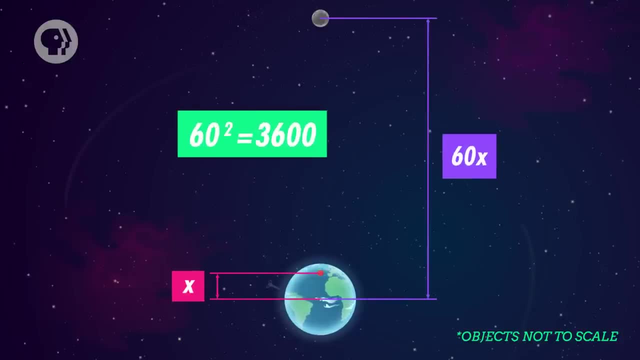 But the Moon has an acceleration that's only about a 3600th of that falling apple. The Moon also happens to be about 60 times as far from the center of the Earth as that apple would be, And 60 squared is 3600.. 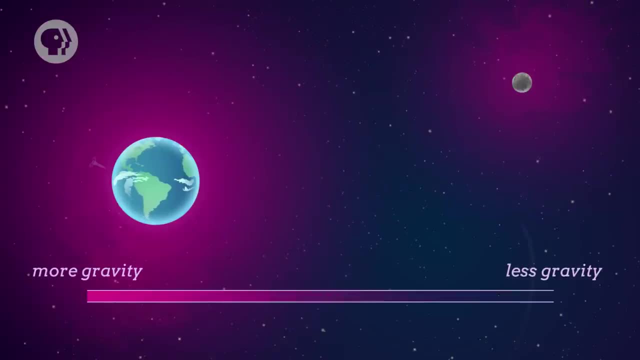 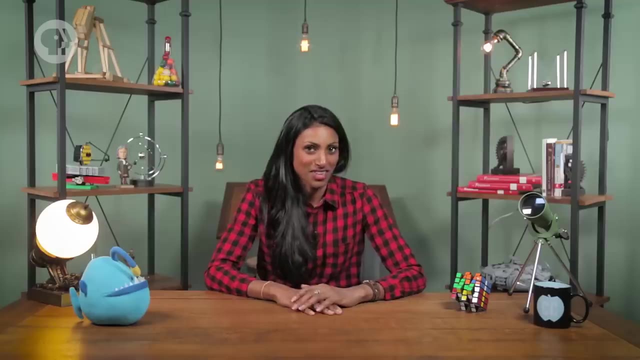 So Newton figured that the gravitational force between two objects must get smaller the further apart they are. More specifically, it must depend on the distance between the two objects squared. Then there was mass, Not the mass of the apple or the Moon, but the mass of the other object involved in the 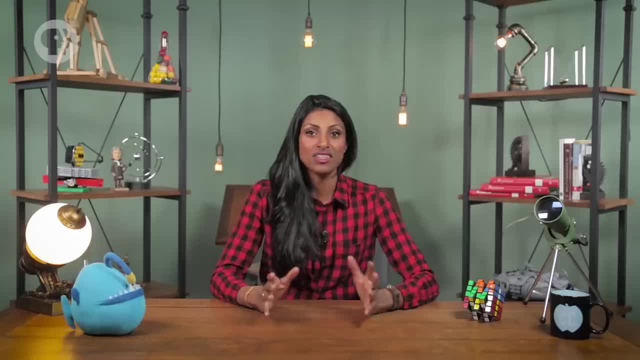 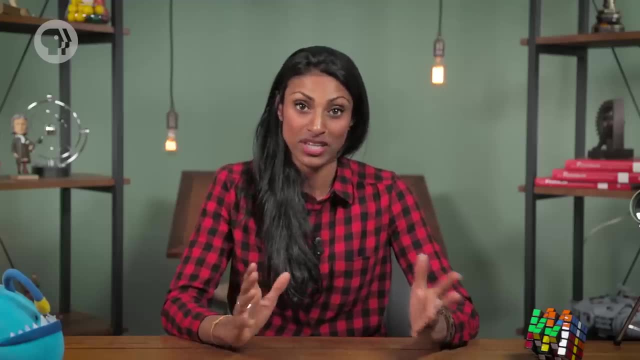 gravitational dance, In this case Earth. Newton realized that the greater the masses of the two objects pulling on each other, the stronger the gravitational force would be between them. Once he had taken into account the distance between two objects and their masses, Newton had most of his equation for the way gravity behaved. The gravitational force was proportional to the mass of the two objects multiplied together, divided by the square of the distance between them. It had to be a lot smaller or else you'd see a force pulling together most everyday. 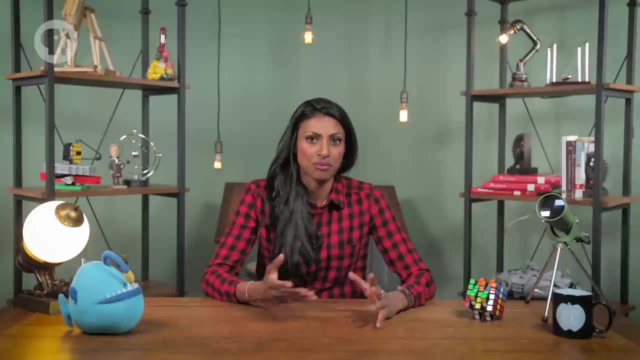 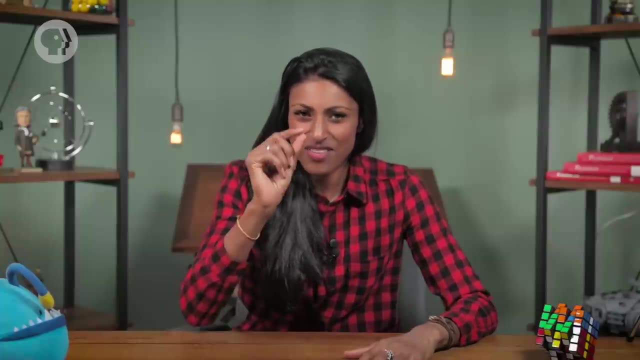 objects Like this Rubik's cube is staying right where it is instead of being pulled towards me. so the gravitational force between us must be very small. So Newton added a constant to his equation, a very small number that would make the gravitational 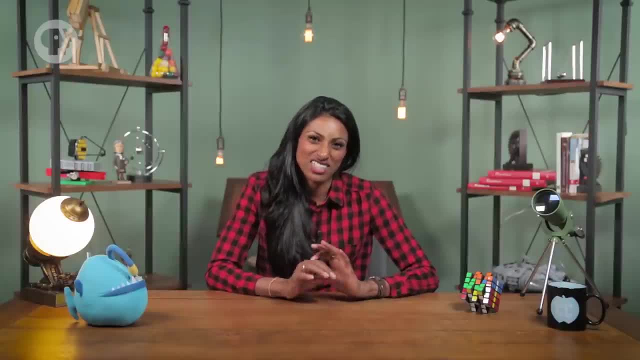 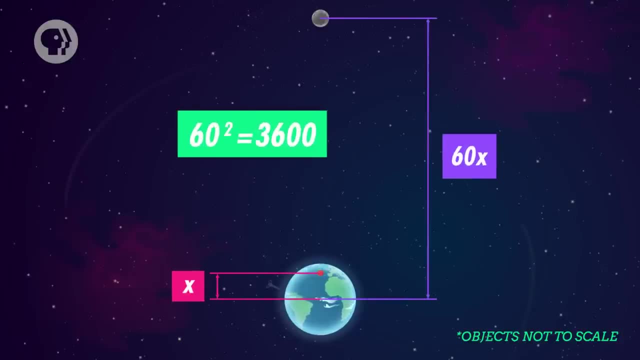 But the Moon has an acceleration that's only about a 3,600th of that falling apple. The Moon also happens to be about 60 times as far from the center of the Earth as that apple would be, And 60 squared is 3,600.. 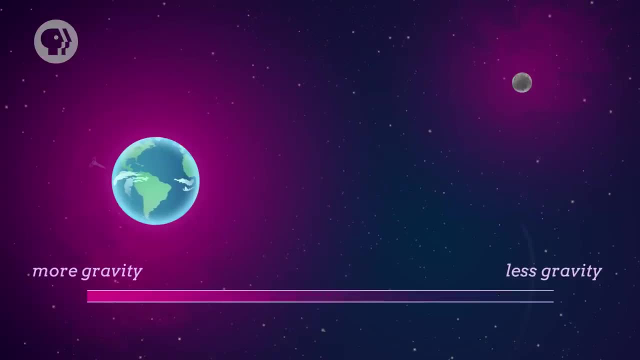 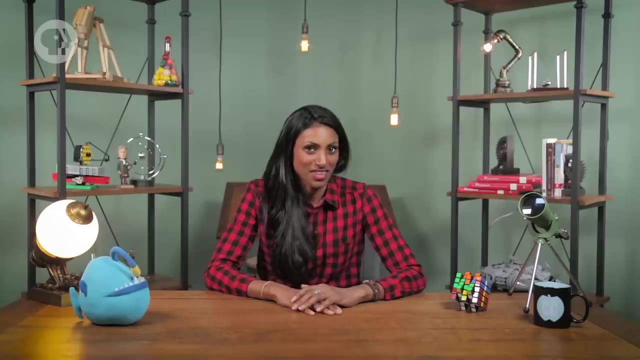 So Newton figured that the gravitational force between two objects must get smaller the further apart they are. More specifically, it must depend on the distance between the two objects squared. Then there was mass, Not the mass of the apple or the Moon, but the mass of the other object involved in the 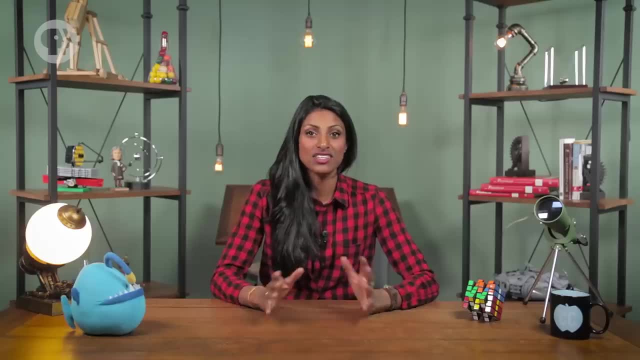 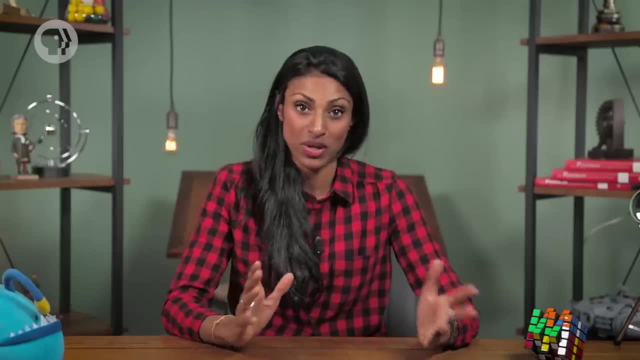 gravitational dance, In this case Earth. Newton realized that the greater the masses of the two objects pulling on each other, the stronger the gravitational force would be between them. Once he had taken into account the distance between two objects and their masses, Newton 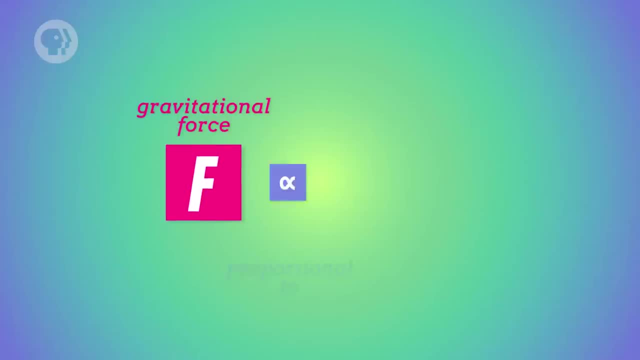 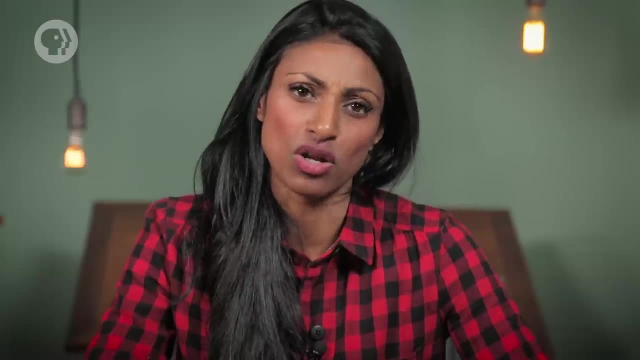 had most of his equation for the way gravity behaved. The gravitational force was proportional to the mass of the two objects multiplied together, divided by the square of the distance between them. It had to be a lot smaller or else you'd see a force pulling together most everyday. 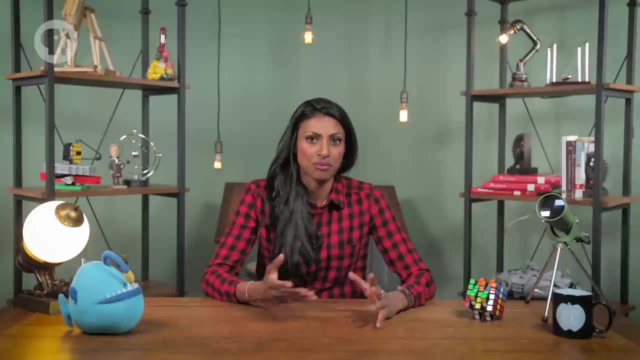 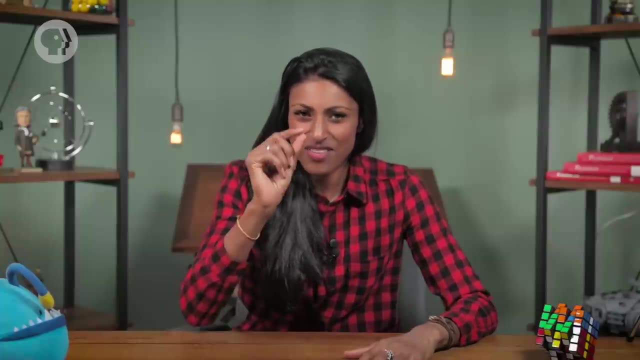 objects Like this Rubik's cube is staying right where it is instead of being pulled towards me. so the gravitational force between us must be very small. So Newton added a constant to his equation, a very small number that would make the gravitational 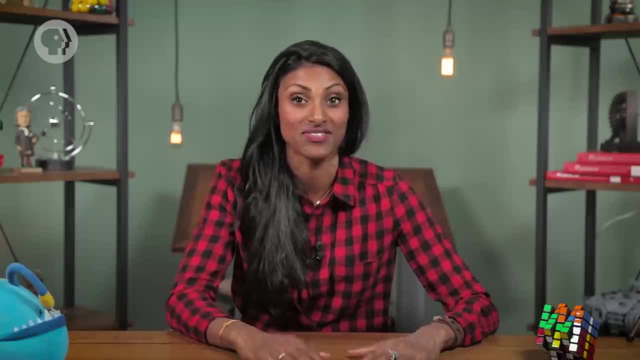 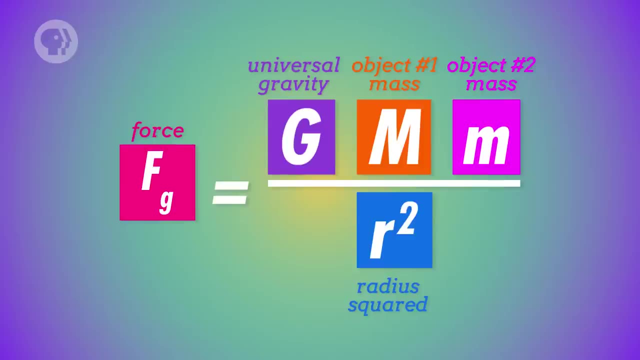 force, just a tiny fraction of what you'd calculate otherwise. He called this a constant, He called it g, And he called this full equation. f equals gmm over r squared the law of universal gravitation. Newton had no idea what number big G would be, though. 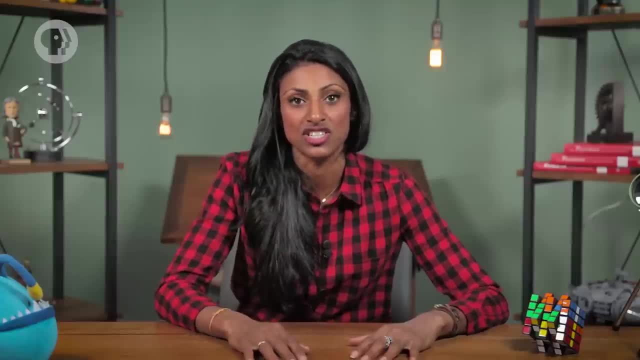 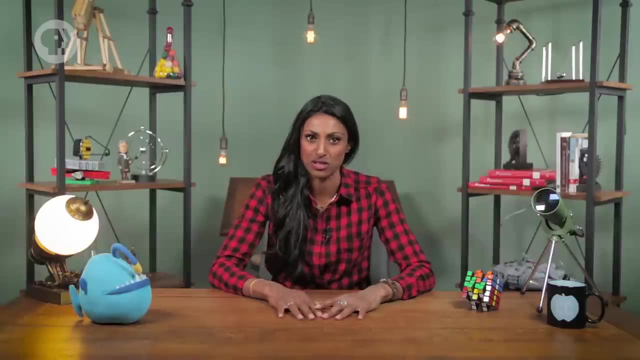 He just knew it would be a tiny number and put the letter g into his equation as a placeholder. About a century later, Henry Cavendish, another British scientist, made careful measurements with some of the most sensitive instruments of the time. He figured out that g was equal to about 6.67 times 10, to the negative 11th newtons times. 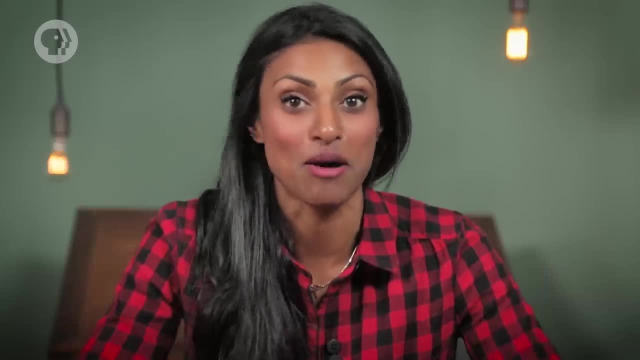 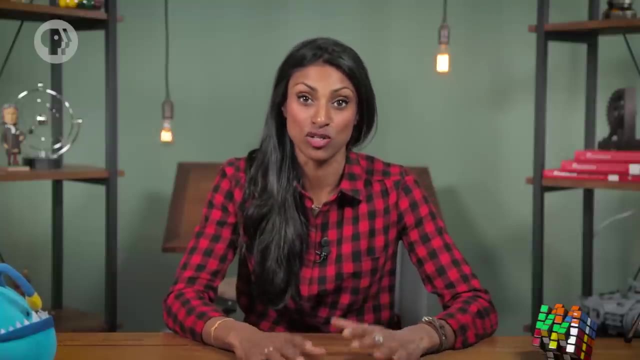 meter squared over kilogram squared. So indeed, Newton was right about big G having to be quite small. But even though he didn't know the exact value of big G at the time, Newton had enough to establish his law of universal gravitation. 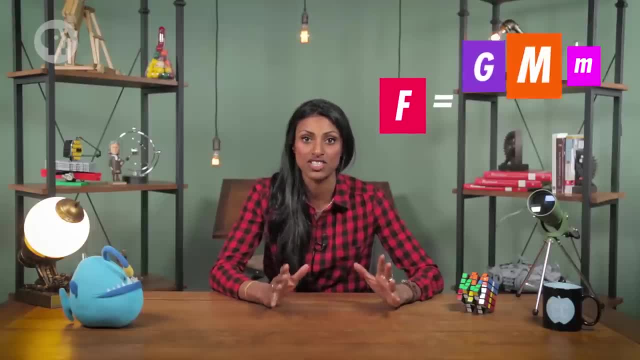 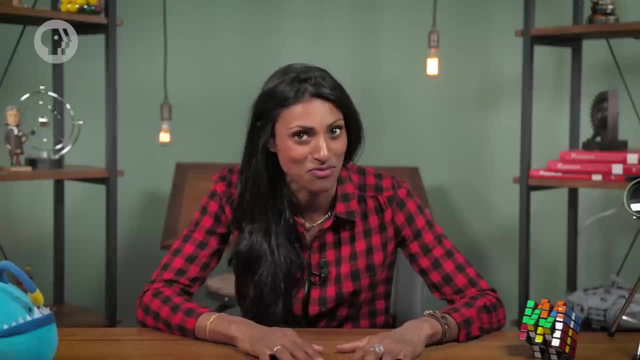 He described gravity as a force between any two objects and published his equation for calculating that force. Then Newton took things a step further, Well, technically three steps further. About 50 years earlier, an astronomer named Johannes Kepler came up with three laws that described the way orbits worked, And those predictions almost perfectly matched the orbits of the universe. So in other words, the law of gravity is the law of gravity. It's the law of the orbits that astronomers were seeing in the sky. So Newton knew that his law of universal gravitation had to fit with Kepler's laws or he'd have to find some other way to explain why Kepler was wrong. Luckily for Newton, his law of gravitation not only fit with Kepler's laws, he was also able to use it in combination with his three laws of motion and calculus to prove. 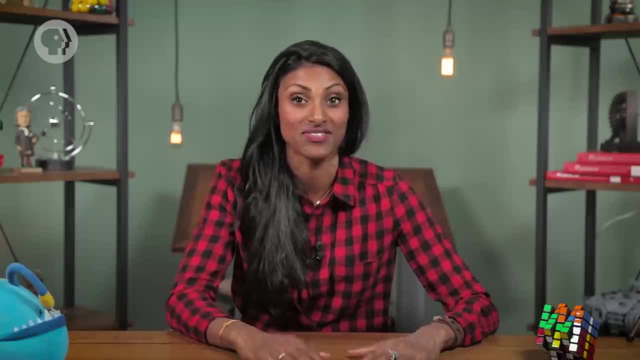 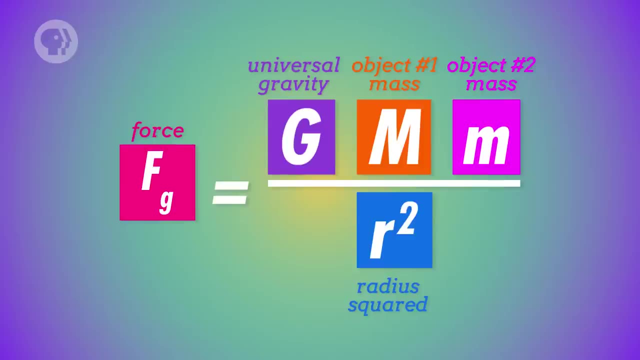 force, just a tiny fraction of what you'd calculate otherwise. He called it g, And he called this full equation: f equals gmm over r, squared the law of universal gravitation. Newton had no idea what number big G would be, though. 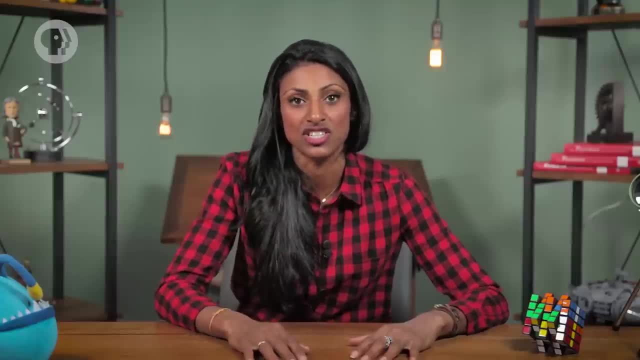 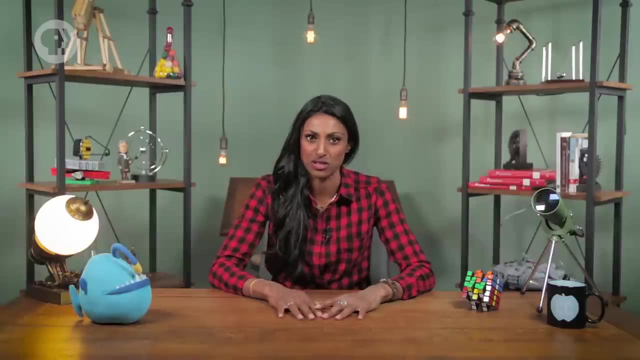 He just knew it would be a tiny number and put the letter g into his equation as a placeholder. About a century later, Henry Cavendish, another British scientist, made careful measurements with some of the most sensitive instruments of the time. He figured out that g was equal to about 6.67 times 10, to the negative 11th newtons times. 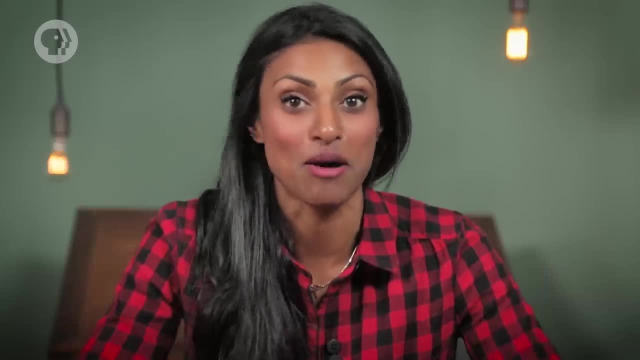 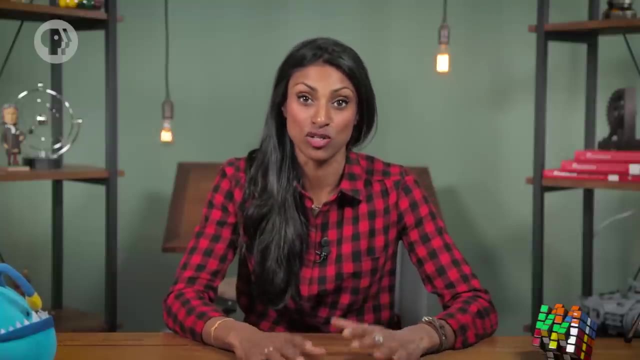 meter squared over kilogram squared. So indeed, Newton was right about big G having to be quite small. But even though he didn't know the exact value of big G at the time, Newton had enough to establish his law of universal gravitation. 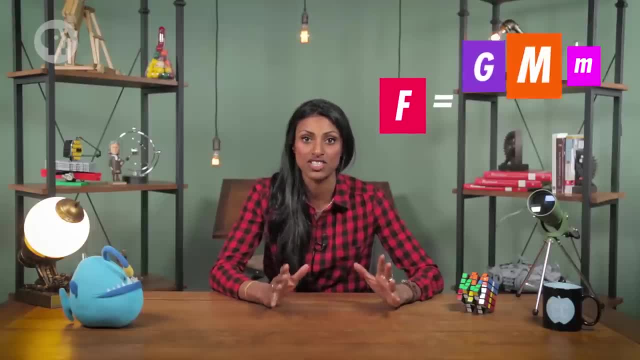 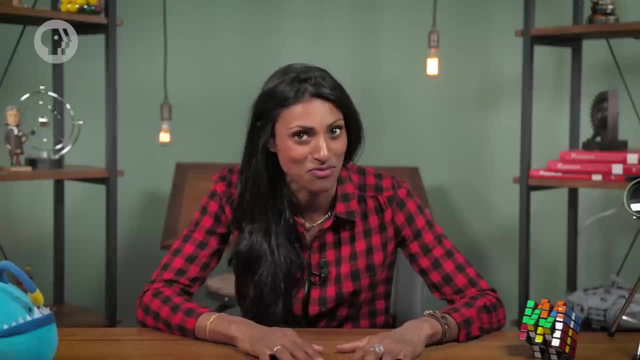 He described gravity as a force between any two objects and published his equation for calculating that force. Then Newton took things a step further, Well, technically three steps further. About 50 years earlier, an astronomer named Johannes Kepler came up with three laws that 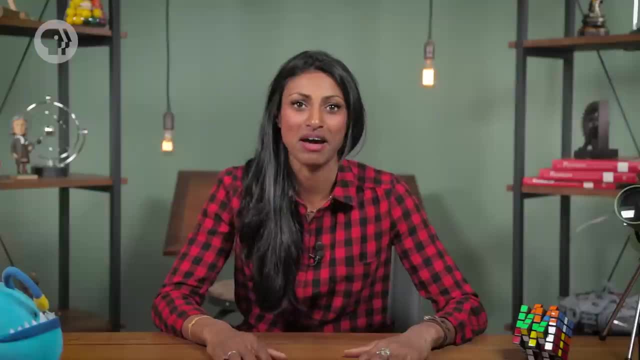 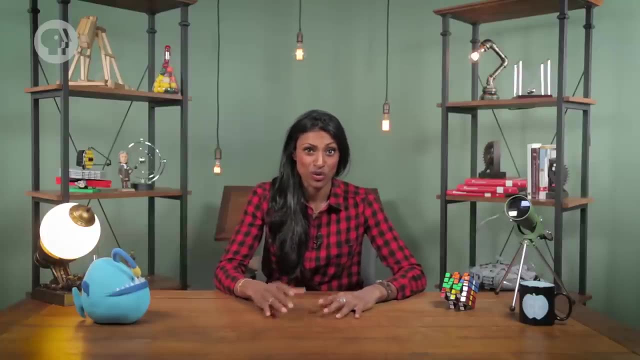 described the way orbits worked, And those predictions almost perfectly matched the orbits that astronomers were seeing in the sky. So Newton knew that his law of universal gravitation had to fit with Kepler's laws or he'd have to find some other way to explain why Kepler was wrong. 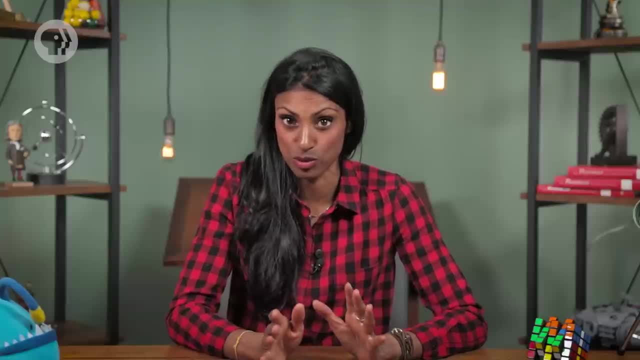 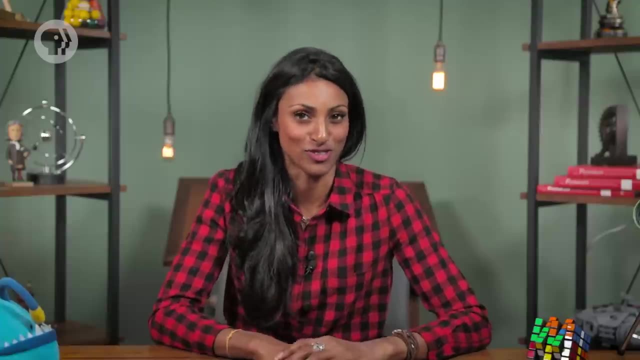 Luckily for Newton, his law of gravitation not only fit with Kepler's laws, he was also able to use it in combination with his three laws of motion and calculus to prove Kepler's laws. According to Kepler, the orbits of the planets were ellipses as opposed to circles, with 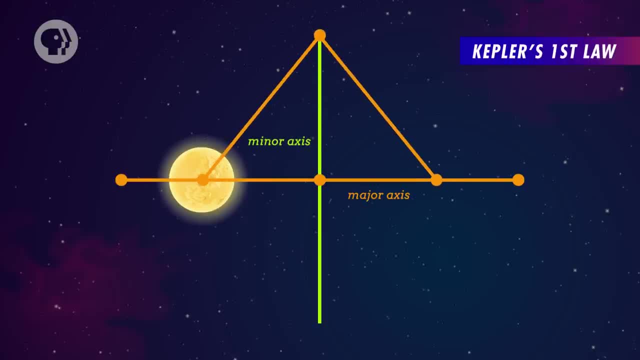 the Sun at one focus of the ellipse. This is one of the two central points used to describe how the ellipse curves, And that's what's known as Kepler's first law, and it actually applies to any elliptical orbit, not just those of planets. 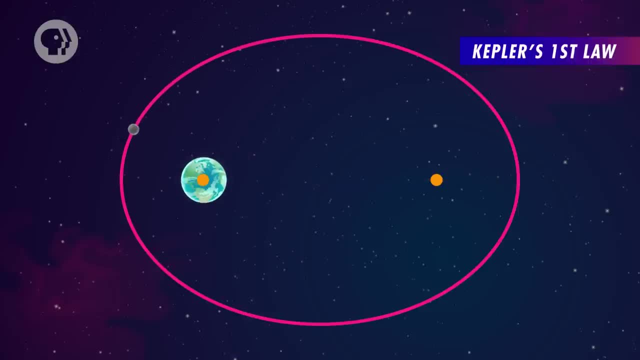 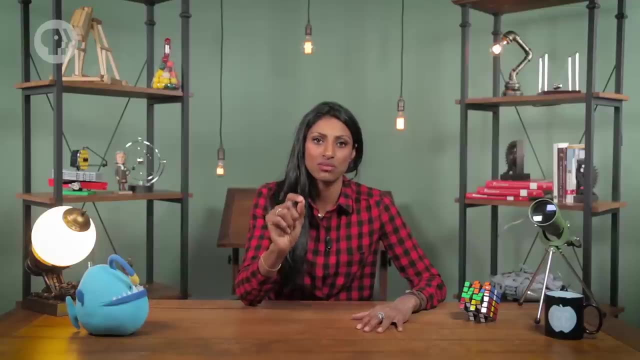 Our Moon's orbit around the Earth is also an ellipse, and Earth is at one focus of that ellipse. Kepler's second law was that if you draw a line from a planet to the Sun, it will always sweep out the same size area within a given amount of time. 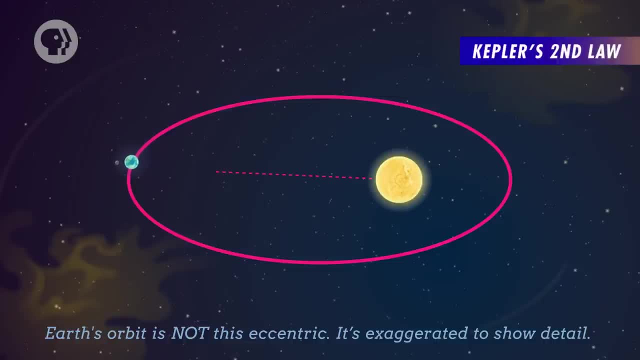 When Earth is at its farthest point from the Sun, for example, over the course of one day we'll have covered an area that looks like a very long, very thin cut-off point. That's Kepler's first law. And when we're at our closest point to the Sun, one day's worth of orbit will sweep. 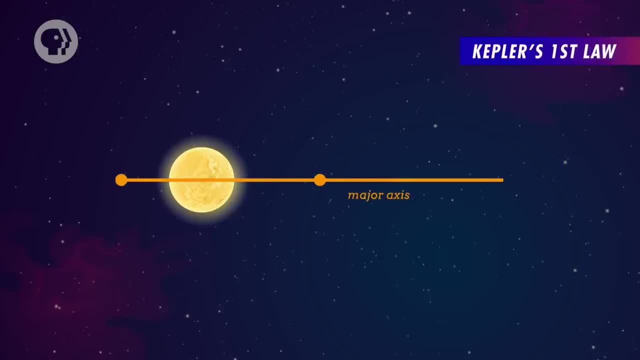 Kepler's laws. According to Kepler, the orbits of the planets were ellipses as opposed to circles, with the Sun at one focus of the ellipse. That's one of the two central points used to describe how the ellipse curves, And that's what's known as Kepler's first law, and it actually applies to any elliptical. 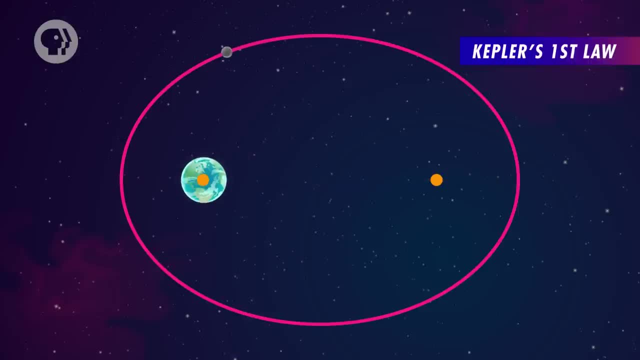 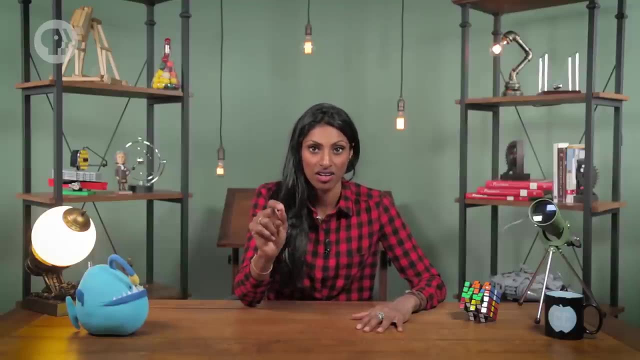 orbit, not just those of planets. Our Moon's orbit around the Earth is also an ellipse, and Earth is at one focus of that ellipse. Kepler's second law was that if you draw a line from a planet to the Sun, it will always. 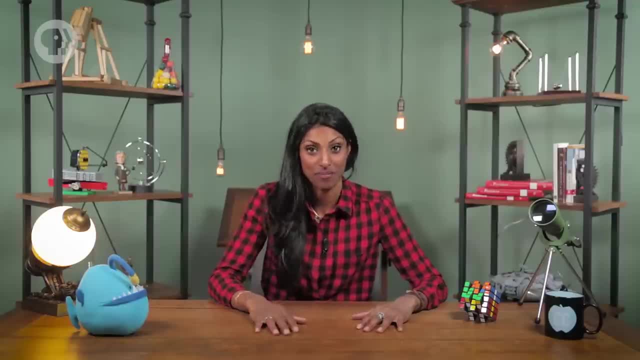 sweep out the same size area within a given amount of time, When Earth is at its farthest point from the Sun, for example, over the course of one day we'll have covered an area that looks like a very long, very thin kind of ellipse. 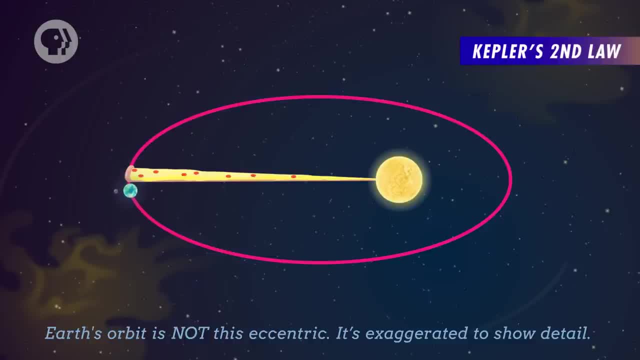 That's Kepler's first law and it actually applies to any elliptical orbit, not just those very thin kind of lopsided pizza slice. And when we're at our closest point to the Sun, one day's worth of orbit will sweep. 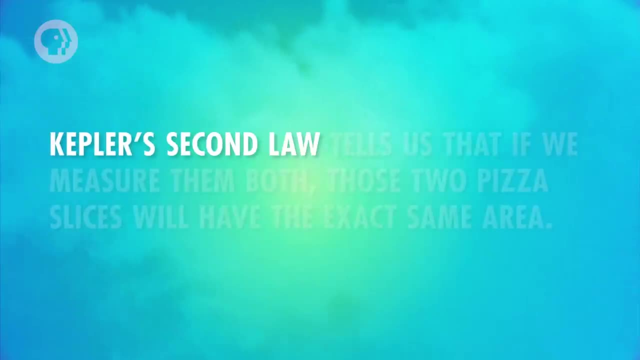 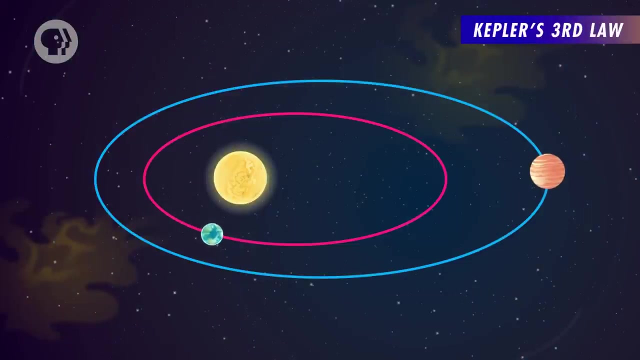 out an area that's more like a short fat pizza slice. Kepler's second law tells us that if we measure them both, those two pizza slices will have the exact same area. His third law is a little more technical, but it's basically an observation about. 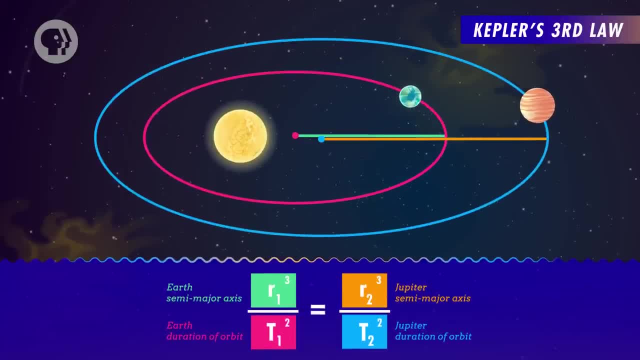 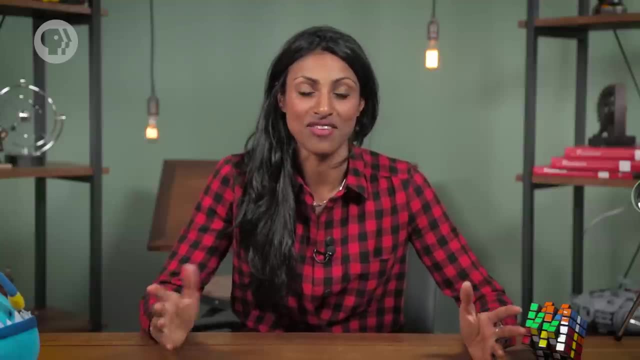 what happens when you take the longest or semi-major radius of a planet's orbit and cube it, then divide that by the period of the planet's orbit squared According to Kepler. that ratio should be the same for every single elliptical orbit. on a single planet, and now we know that it is Almost exactly. For every single planet that orbits our Sun, that ratio is either 3.34 or 3.35.. And Newton was able to explain why the actual observed orbits in the night sky sometimes deviated very slightly from Kepler's predictions, For example by having those slightly different ratios. What Kepler didn't know and Newton figured out was that the planets and moons were all pulling on each other, and sometimes that pull was strong enough to change their orbits. 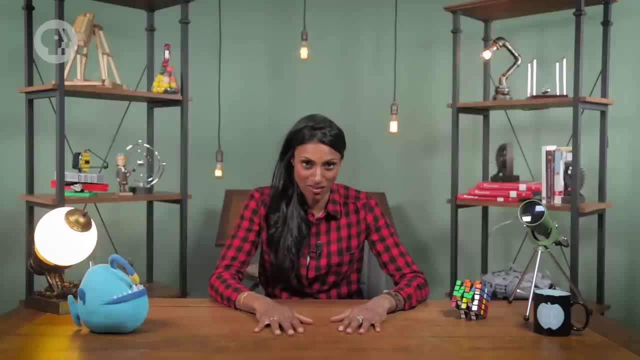 just a little bit. There's one more thing we should point out. There's one more thing we should point out about the law of universal gravitation, which is that it fits what we expect the equation for a net force to look like, according to. 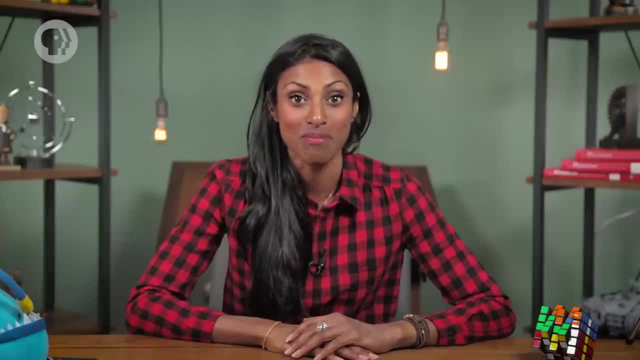 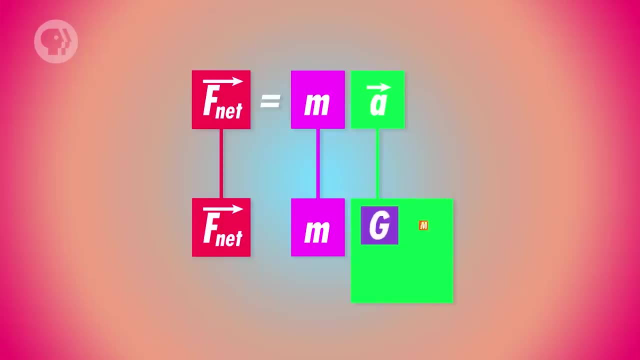 Newton. From Newton's second law of motion we know that a net force is equal to mass times acceleration. What the law of universal gravitation is saying is that when the net force acting on an object comes from gravity, the acceleration is equal to the mass of the bigger object, like Earth. 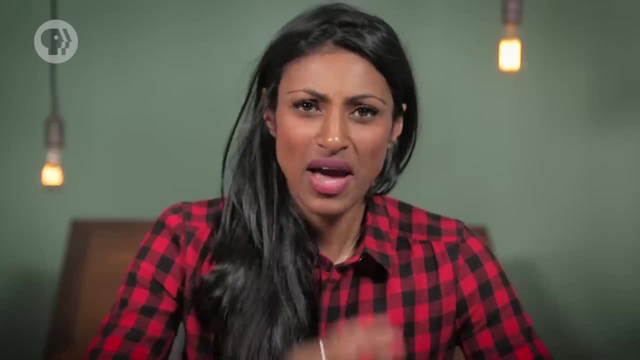 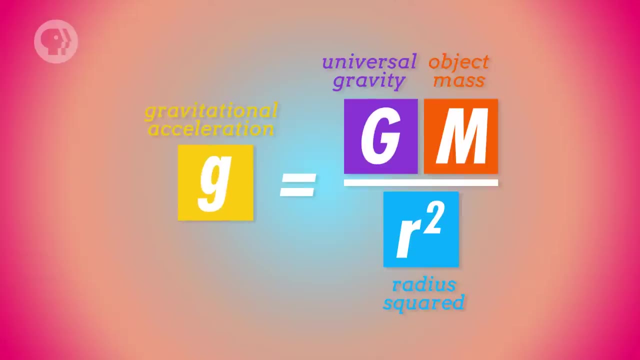 divided by the distance between the two objects times big G. So you know how we've been describing the gravitational acceleration at Earth's surface as small g. Well… It's equal to big G times Earth's mass divided by Earth's radius squared. 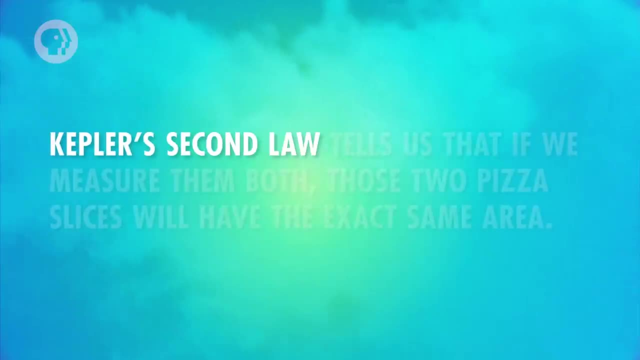 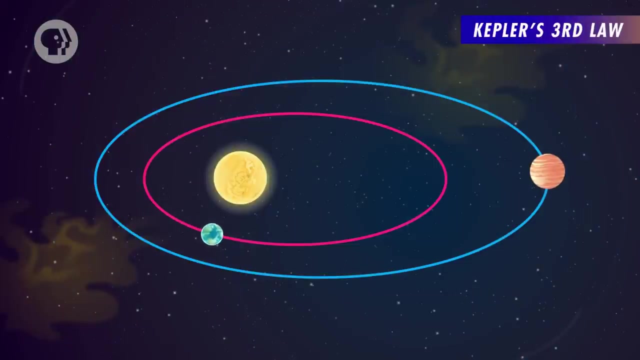 out an area that's more like a short fat pizza slice. Kepler's second law tells us that if we measure them both, those two pizza slices will have the exact same area. His third law is a little more technical, but it's basically an observation about. 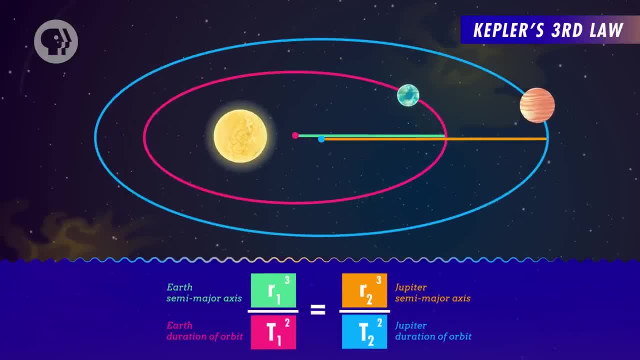 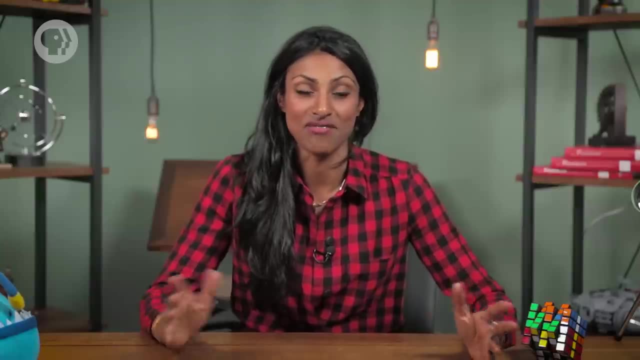 what happens when you take the longest or semi-major radius of a planet's orbit and cube it, then divide that by the period of the planet's orbit squared According to Kepler. that ratio should be the same for every single planet. And now we know that it is Almost exactly. For every single planet that orbits our Sun, that ratio is either 3.34 or 3.35.. And Newton was able to explain why the actual observed orbits in the night sky sometimes deviated very slightly from Kepler's predictions. 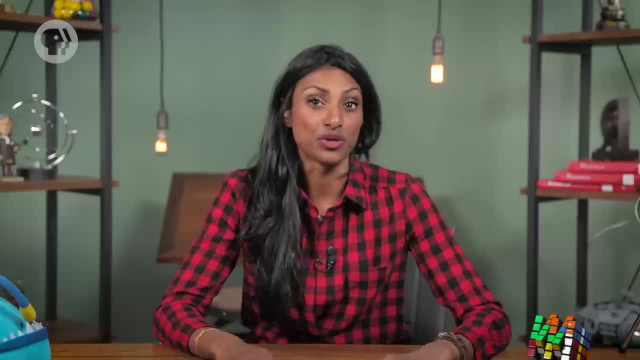 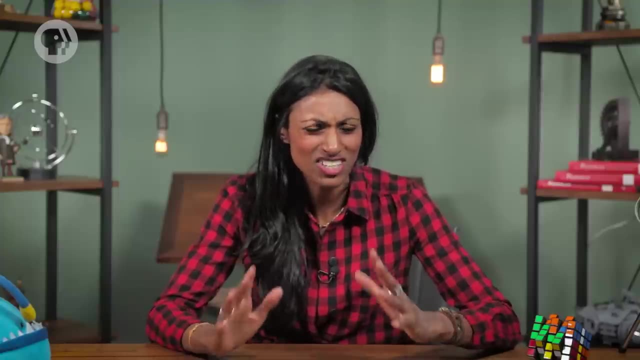 For example, by having those slightly different ratios. What Kepler didn't know and Newton figured out was that the planets and moons were all pulling on each other, and sometimes that pull was strong enough to change their orbits just a little bit. There's one more thing we should point out about the long-term orbit. 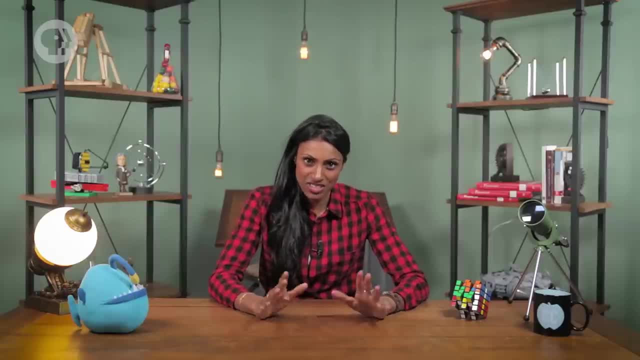 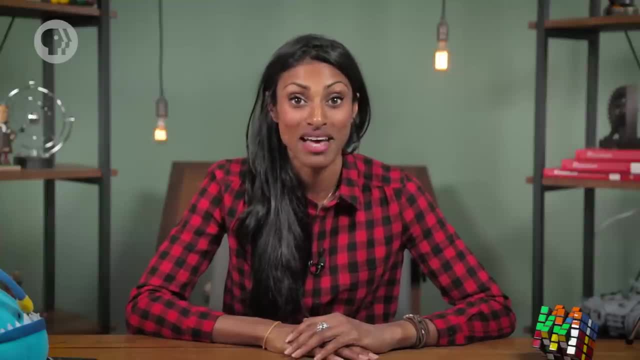 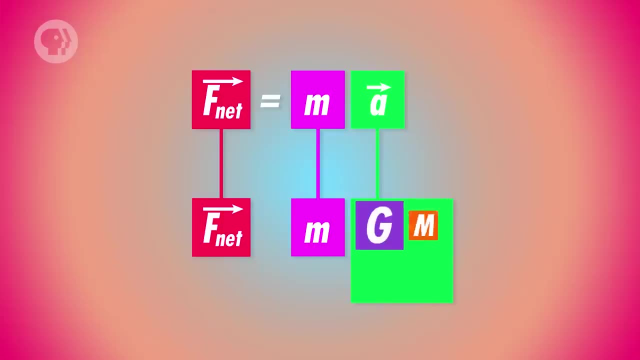 Newton. From Newton's second law of motion we know that a net force is equal to mass times acceleration. What the law of universal gravitation is saying is that when the net force acting on an object comes from gravity, the acceleration is equal to the mass of the bigger object, like Earth. 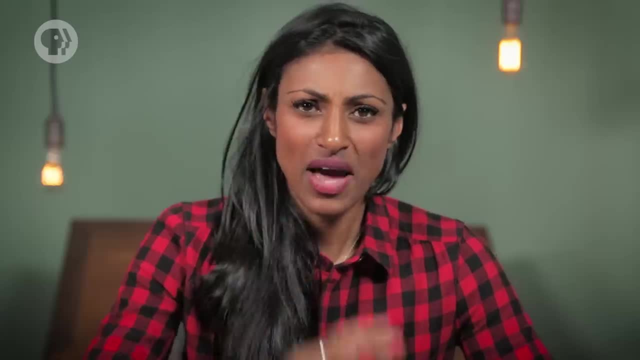 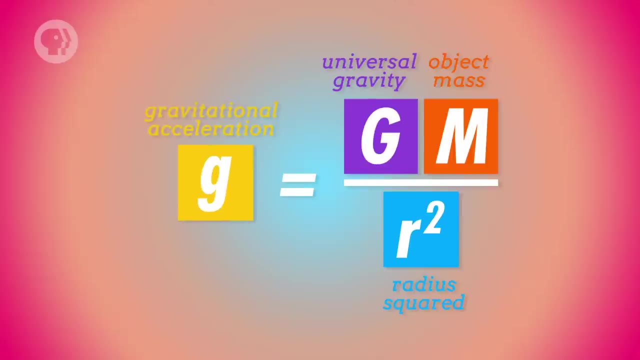 divided by the distance between the two objects times big G. So you know how we've been describing the gravitational acceleration at Earth's surface as small g. Well, small g is actually equal to big G. Big G times Earth's mass divided by Earth's radius squared. 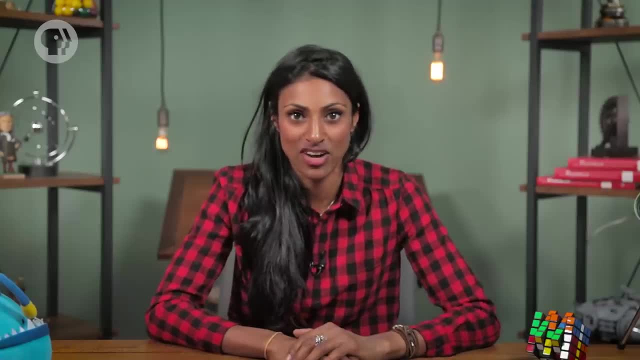 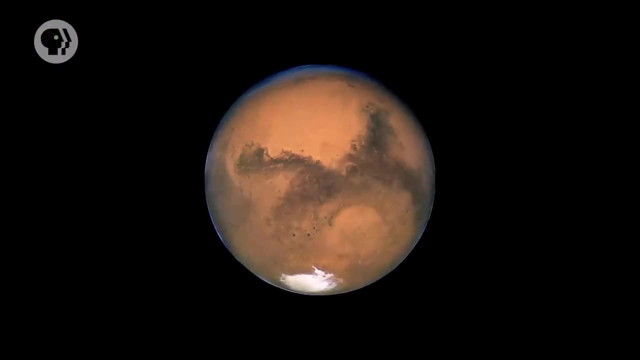 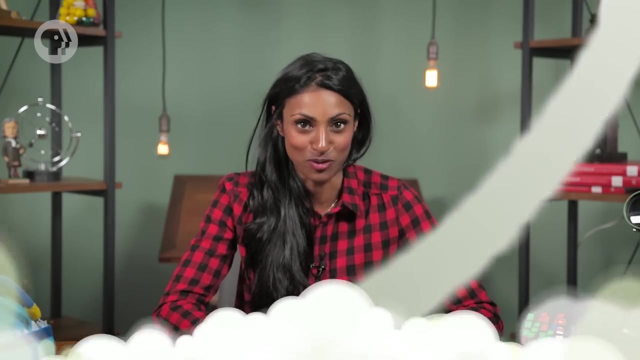 Math, And we can use this equation for gravitational acceleration to help NASA out with a challenge they're grappling with right now. We want to send humans to Mars, but we have to make sure their spacesuits will work properly in Martian gravity. One way that NASA tests spacesuits is by flying astronauts on special planes, sometimes called. 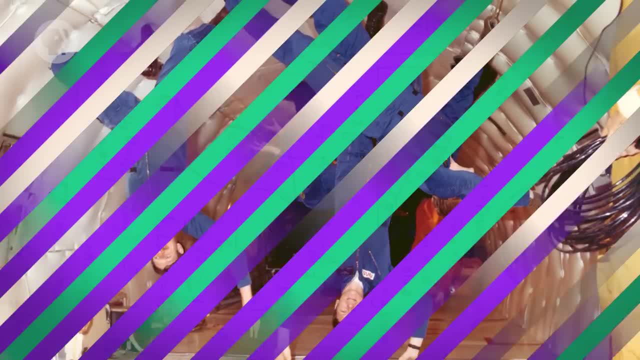 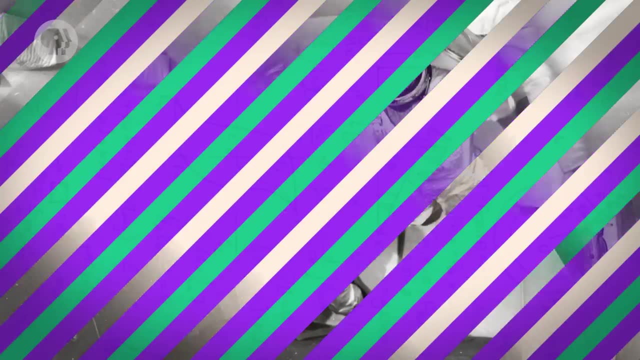 vomit comets. They fly in arcs that let the spacesuit testers experience reduced weight or none at all for short periods of time. To simulate Martian gravity, a flight plan will need to aim for the gravitational acceleration you'd experience if you started. 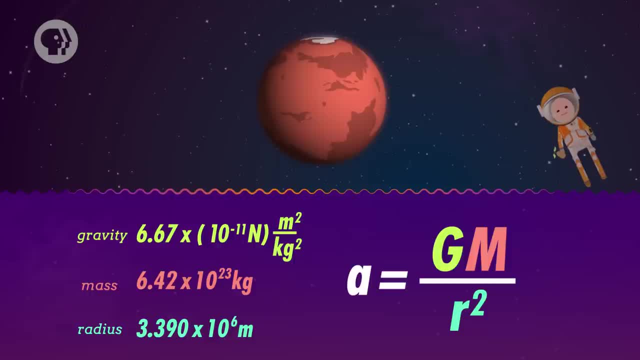 hopping around on the surface of Mars. So what would that acceleration be? Well, from Newton's law of universal gravitation we know that the acceleration of stuff at Mars' surface would be equal to big G times the mass of Mars divided by Mars' radius. 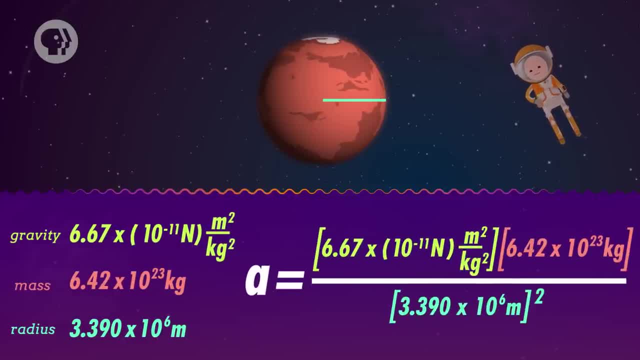 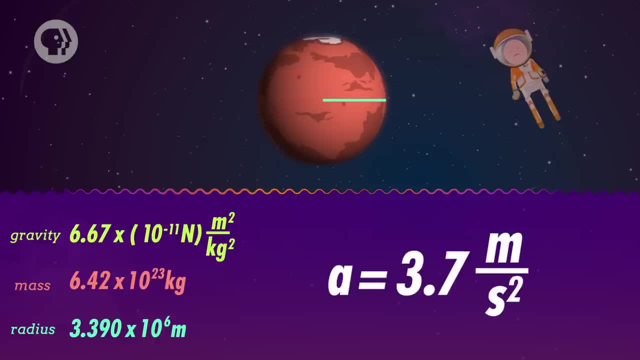 squared. We also happen to know Mars' mass and radius already, Which helps. So, plugging in the numbers, we can calculate the gravitational acceleration at Mars' surface. It should be about 3.7 meters per second. That's a lot.